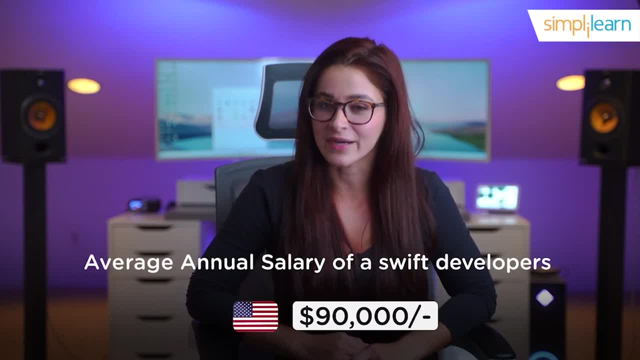 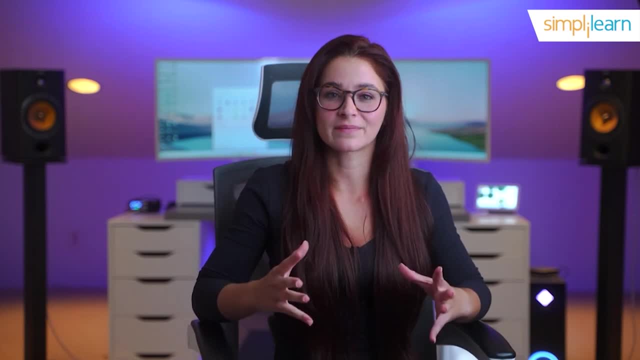 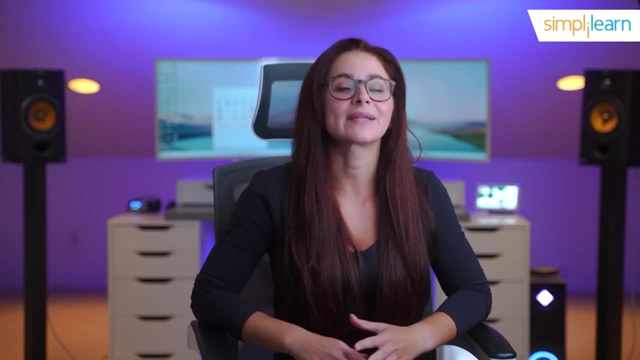 developers bag about $90,000 per annum in America. Up ahead we have C and C++, the humble languages of the entire clan of programming. C is titled the mother of all programming languages. The veteran programming language has contributed a lot to developing new languages compilers. 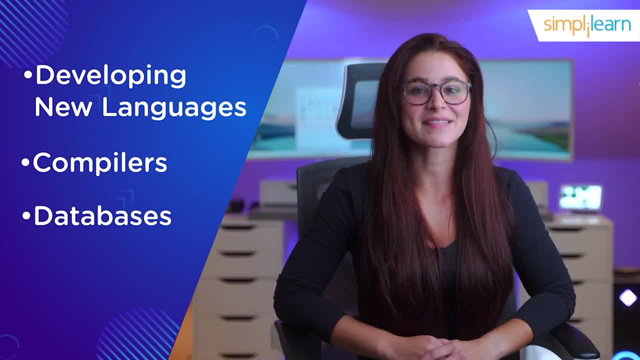 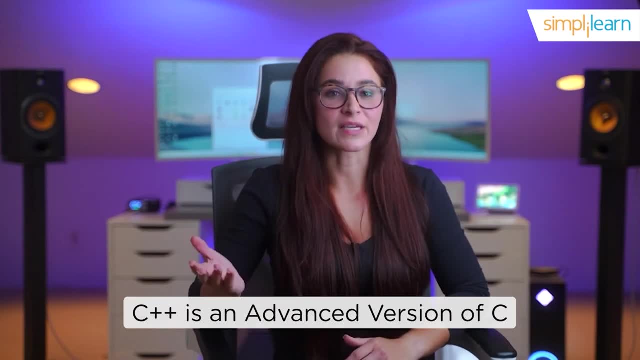 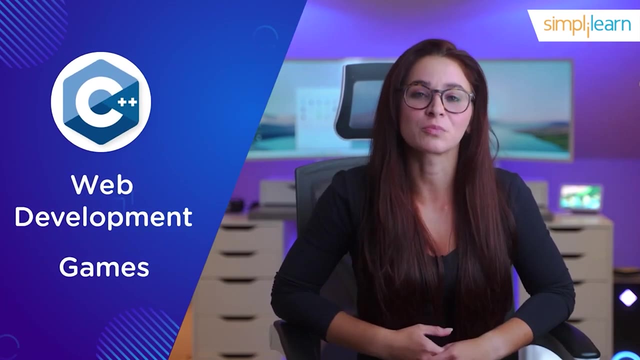 databases and one of the most popular operating systems, Microsoft Windows. On the other hand, C++ is an advanced version of C with object-oriented programming abilities. C++ is used for web development, games and much more. Companies like Microsoft, Netflix and many more use these programming languages. 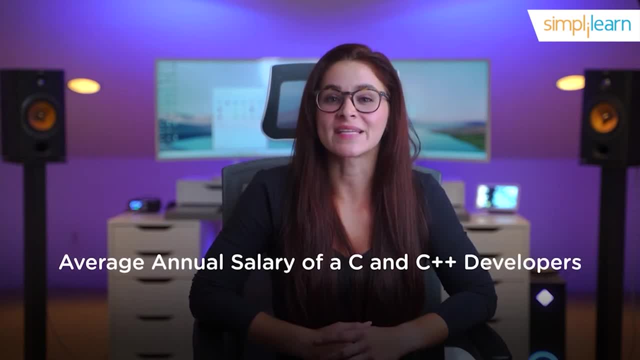 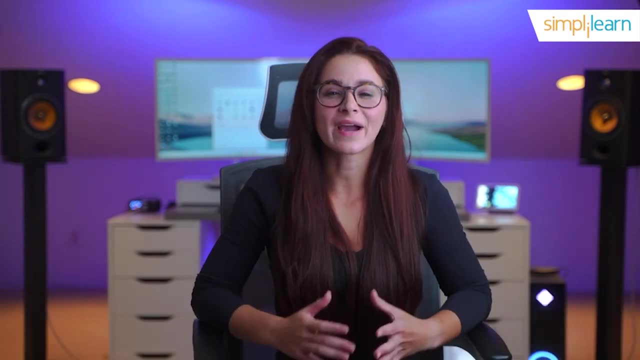 The average salary of C and C++ developers in India is 10 lakhs per annum. In the USA, the salary is $120,000 per annum. Next, we have the top three programming languages you've been waiting for. At three, we have JavaScript. 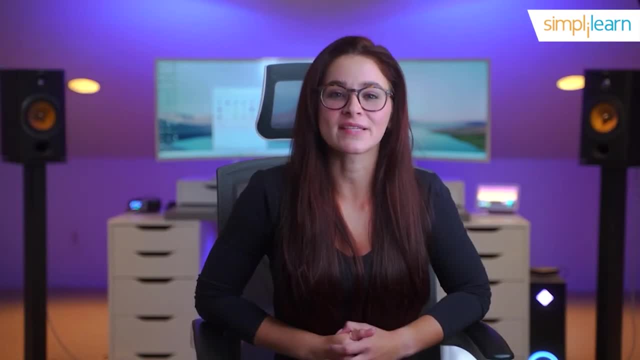 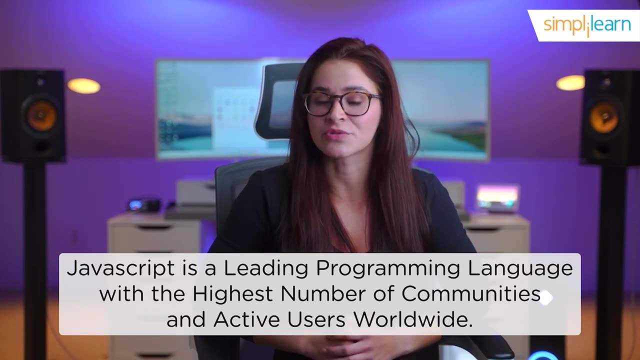 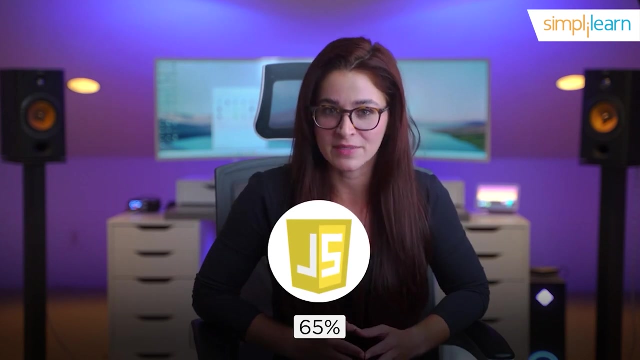 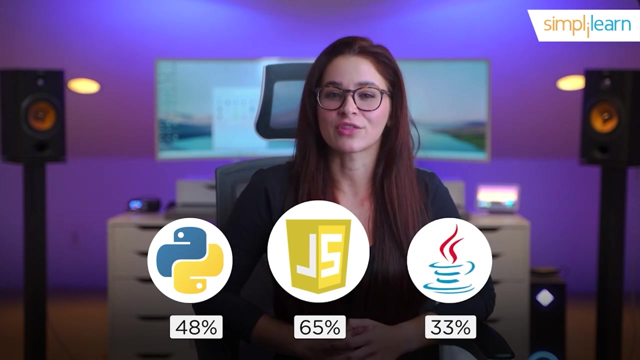 The most versatile and powerful language that turned the face of the internet. JavaScript is a leading programming language with the highest number of communities and active users worldwide. An astonishing number of 65% of programmers around the world use JavaScript. Sharing the podium are Python, with 48% in the second, and Java, with 33% in the third. 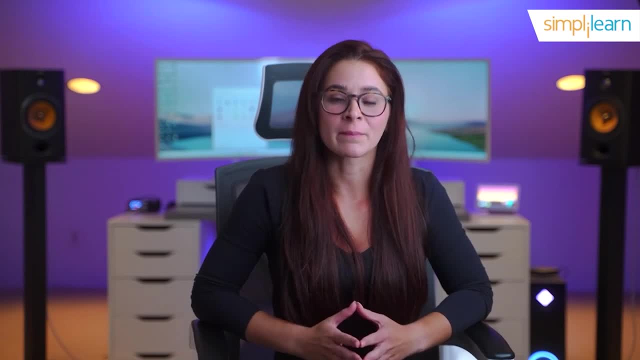 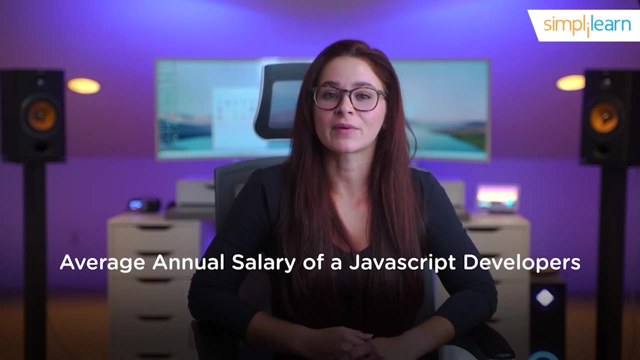 Java Script is used majorly for web development by companies like Netflix, Google, Paypal, BigBasket and more. The salary of a Javascript developer in India is 1,600,000 per annum and in the USA the salary is $135,000 per annum. At number two, we have Java. Java is invincible among all languages. Java has the largest community repositories and support support. It has spread its roots into every software framework: mobile application, big data and operating system. You name it Java, did it? IT giants like Meng and many other IT firms use Java. The salary of a Java developer. 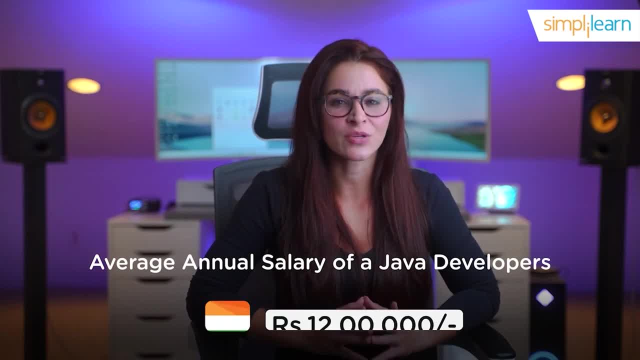 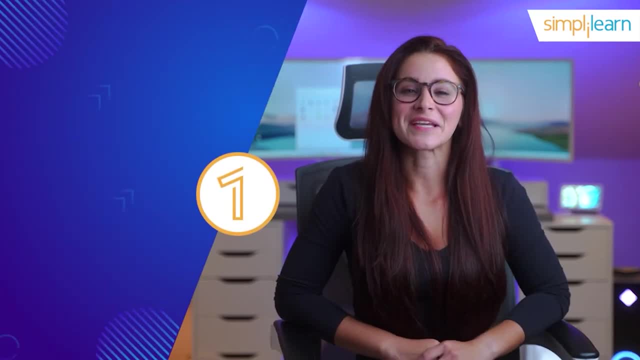 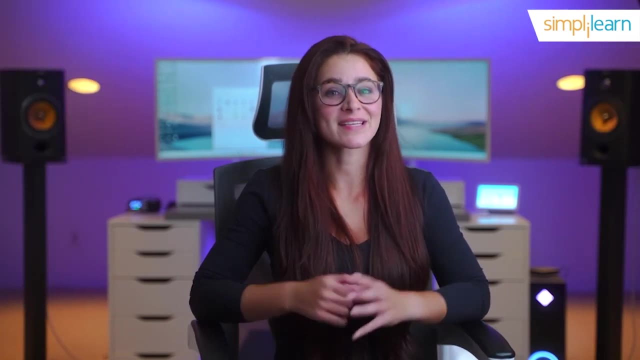 in India is 1 million 200 thousand per annum and in the USA the salary is a hundred twenty thousand dollars per annum. Finally, our number one programming language is Python. Many believe that Python is one of the newest programming languages. As a matter of fact, it's a veteran programming language that is a